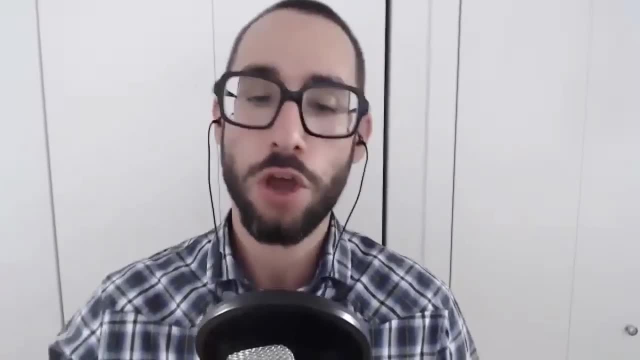 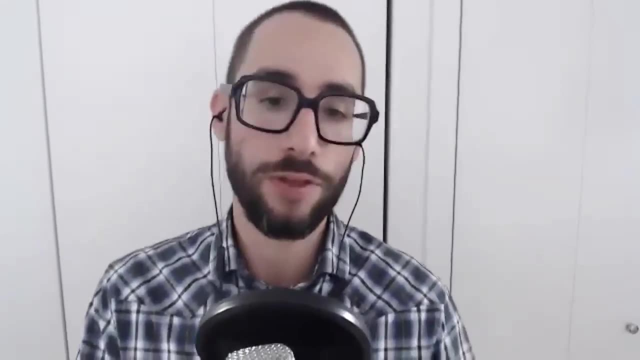 For those who haven't seen it, if you go on familiarlsacorg you can play around with the familiarization tool. There's tests 71,, 73, and 74 on there. There will be a few more in the near future. But as far as the tools, I don't love them, I wouldn't use them. I would say 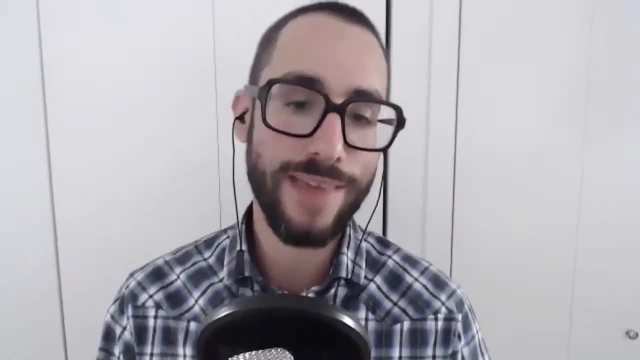 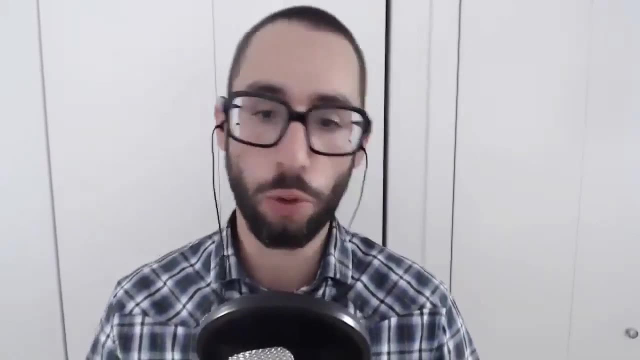 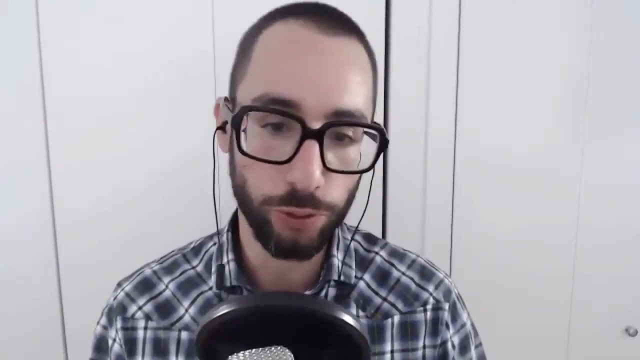 just stick with your scratch paper, Have. that be all you need. You write down a few key words, a few key phrases, Maybe for reading comprehension. of course it's more useful to do little summaries or phrase summaries For logical reasoning. I don't think it's necessary or useful at all, though. 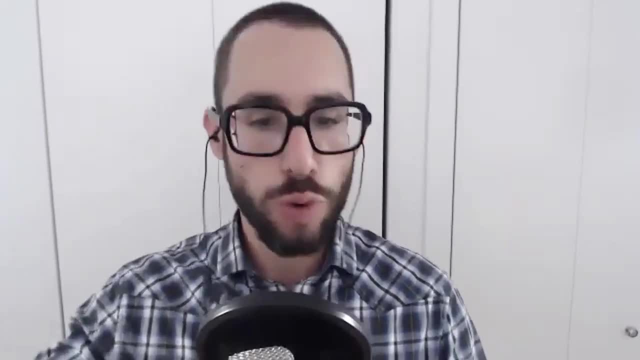 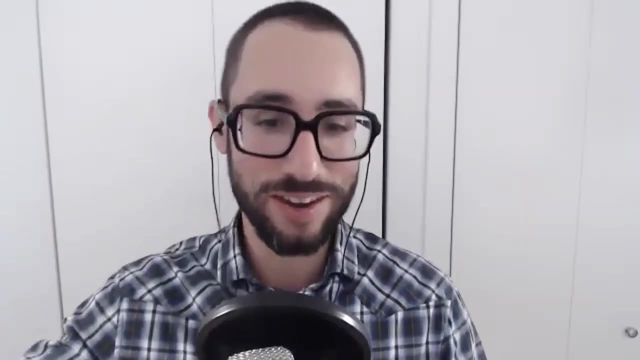 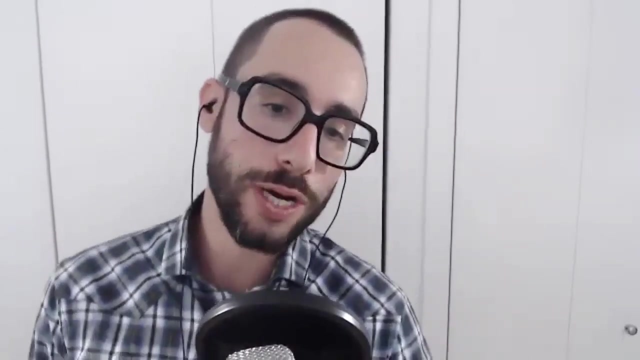 One thing you might do is highlight, in between the evidence and conclusions, You could highlight if there's a period that ends the evidence sentence and then right before the conclusion sentence, you could highlight that little period as kind of making a separation, Or you could. 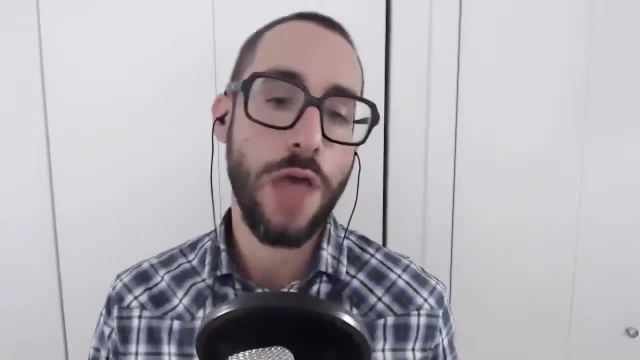 highlight a little period that ends the evidence sentence and then right before the conclusion sentence. you could highlight that little period as kind of making a separation. Or you could highlight a key word or phrase in the question stem. that relates to the question type, But I 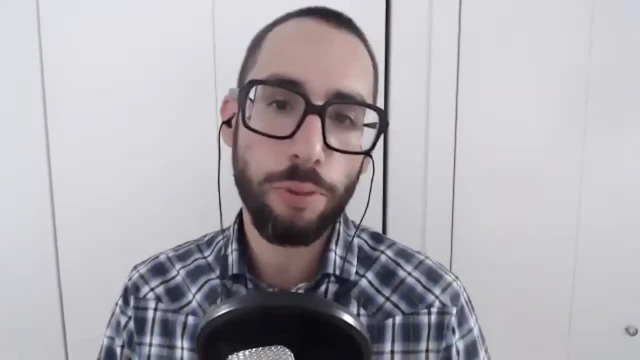 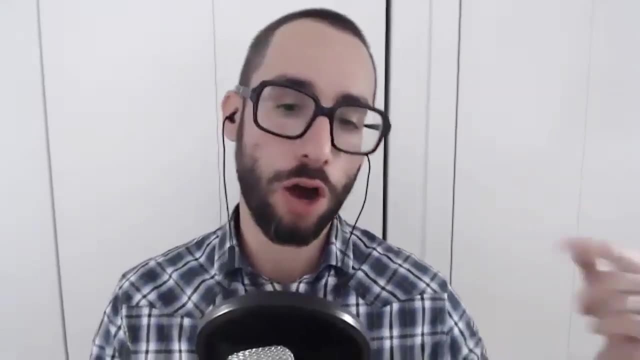 wouldn't do more than that, And I certainly wouldn't do it for reading comprehension either. Pre-phrasing is actually more about engaging with the method of reasoning and being familiar with the underlying general principle. To me, it's not about question type, The only way in which it does. 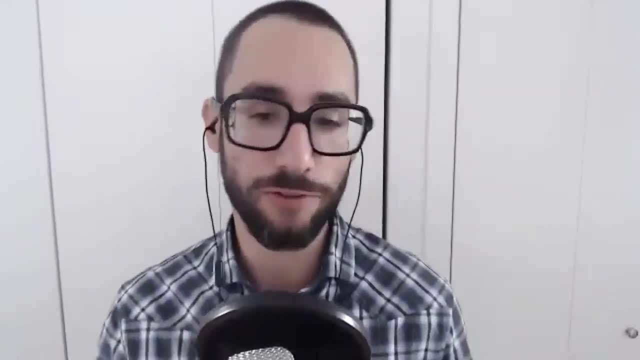 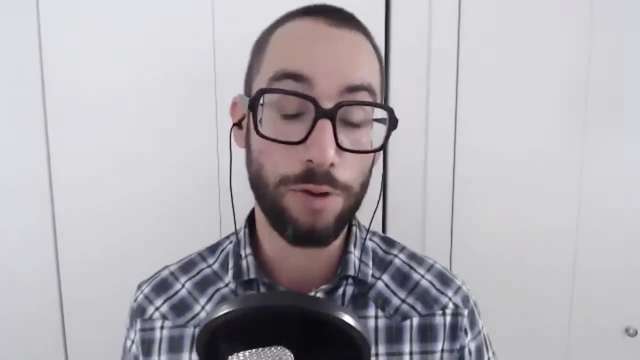 relate to question type in my mind is that certain question types lend themselves to pre-phrasing and others don't. For flaw questions you can definitely pre-phrase if you can articulate and identify the flaw for yourself. But for inference questions there are multiple potential. 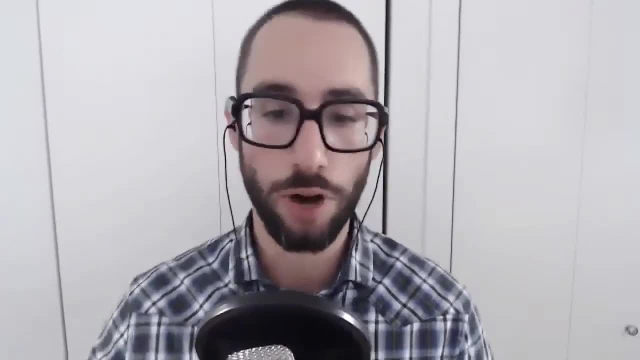 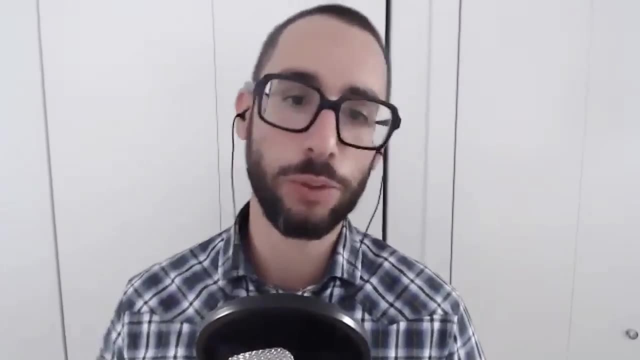 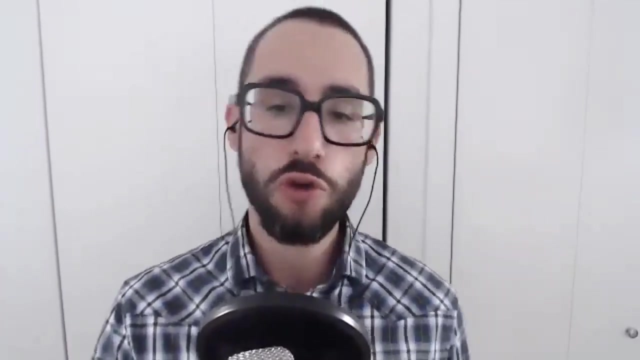 inferences and you don't always know where they're going to draw from, But for me, the predictions. it comes back to engaging with the method of reasoning, engaging with the argument in a very real world sense, as if somebody was having a conversation with you. So the more that. 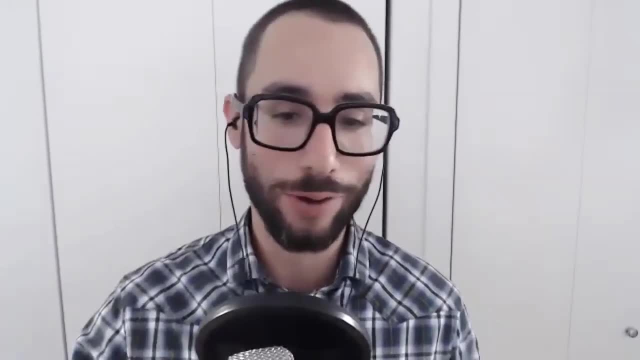 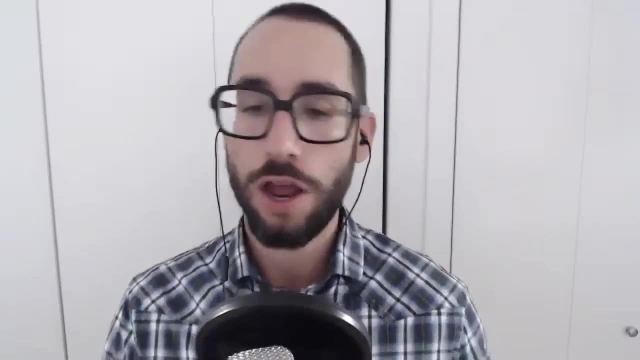 you can do that, and the more you can get away from the abstract language and make it relatable, the better off you'll be, The faster you'll relate to it. And so, as an exercise, if you're seeing tough language- whether it's in the stimulus, like a topic on aestheticism- for me was always like a very